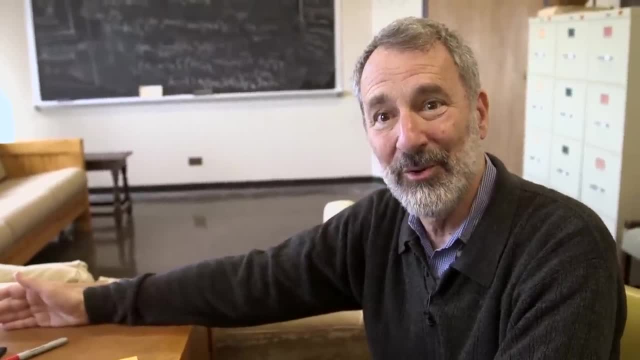 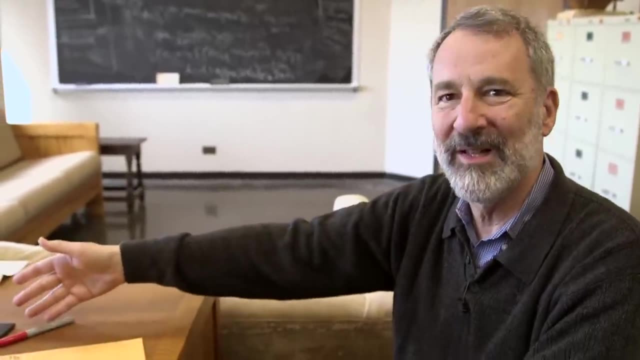 but that sum will be more than 50 trillion. That's true not only for 50 trillion, but for any number you name, no matter how big, and that's what it means: that the sum of the series is infinity. So it's blowing up. It's like, exactly, it's getting away from us. Exactly, We say that. 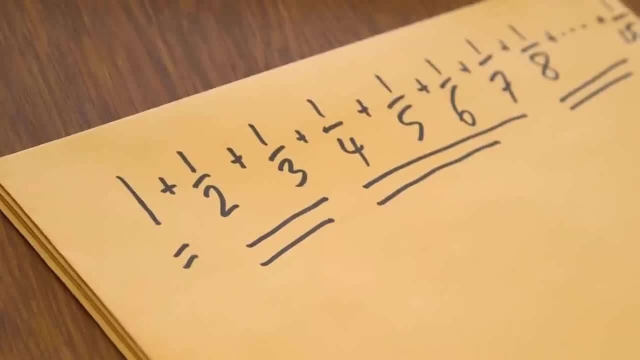 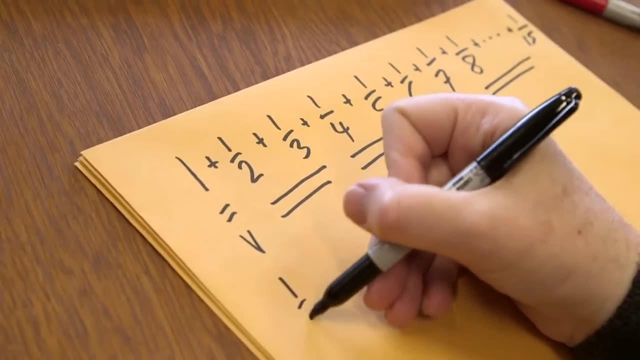 the sum of the series diverges. So let's look at the first term. Well, it's one, Thank you. How about these next two terms? Well, you know what. this one is bigger than a half. Each one of these terms is bigger than a quarter. A half is bigger than a quarter. A third is bigger. 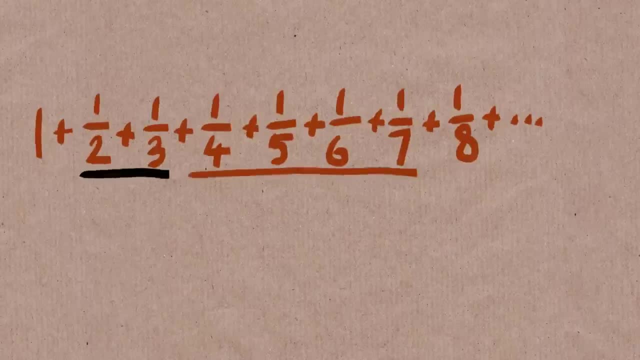 than a quarter and there are two terms. So this is bigger than two quarters, which is again a half. How about these four terms? They're all bigger than one-eighth and there are four of them, So if I add these guys, it's one-eighth. 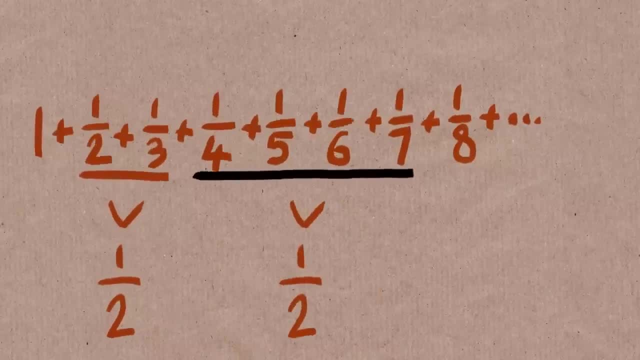 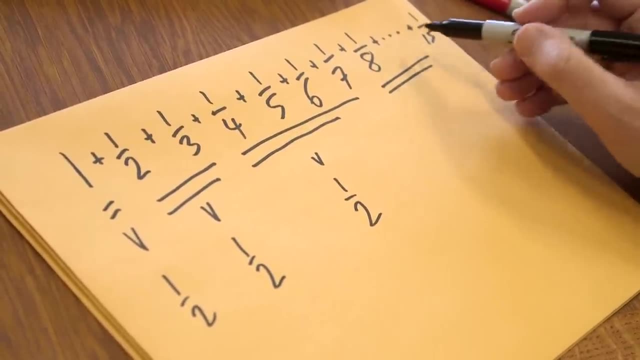 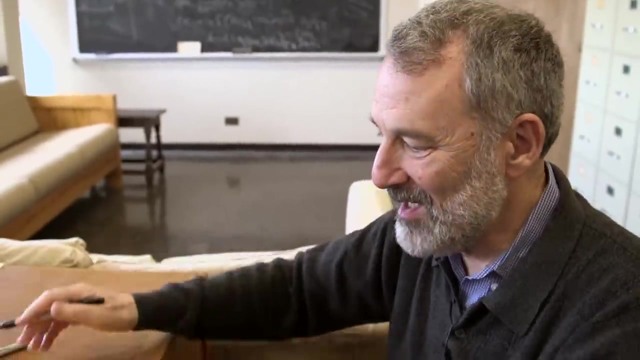 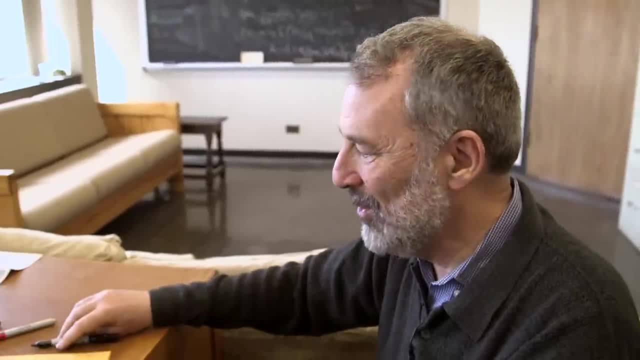 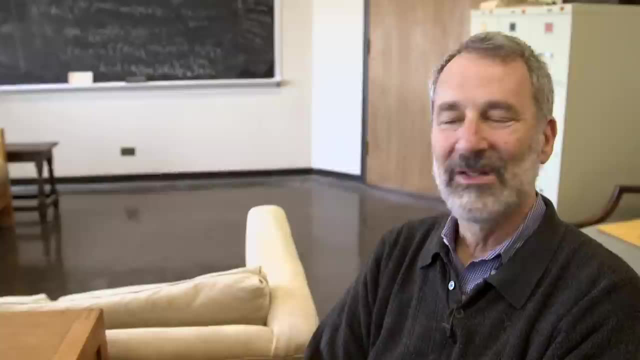 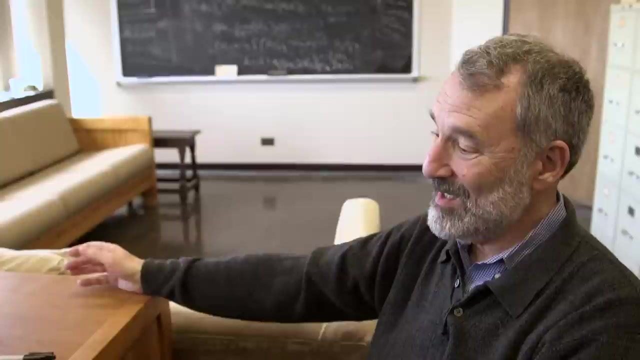 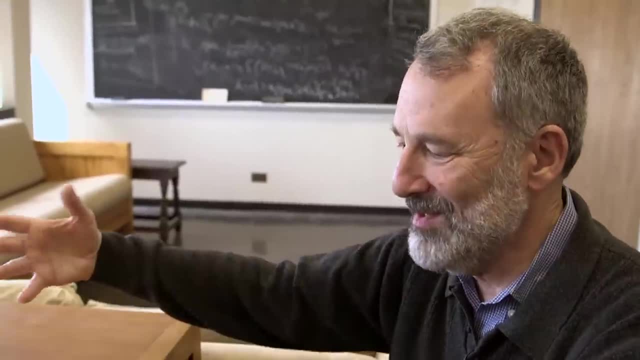 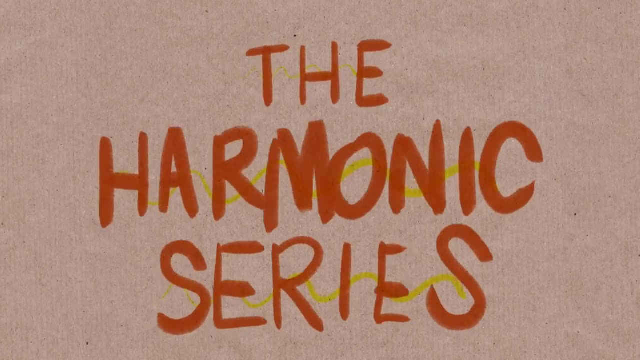 not worry about that now. Okay, never mind just how enormous, Let's leave it there. for this sum which has a name, It's called the harmonic series. I'd like to explain how to use the harmonic series to stack dominoes. Well, actually, I'm going to explain how to use the harmonic series to stack dominoes. Well, actually, I'm going to explain how to use the harmonic series to stack dominoes. Well, actually, I'm going to explain how to use the harmonic series to stack dominoes. Well, actually, I don't have dominoes. 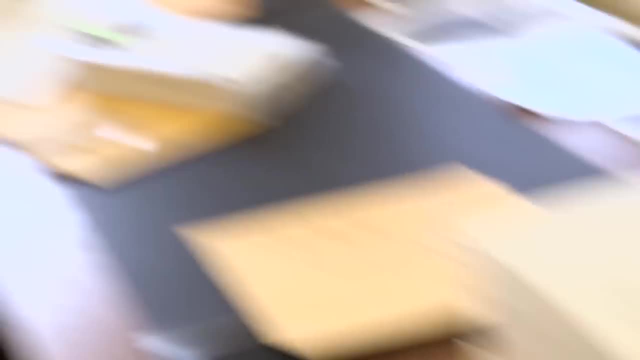 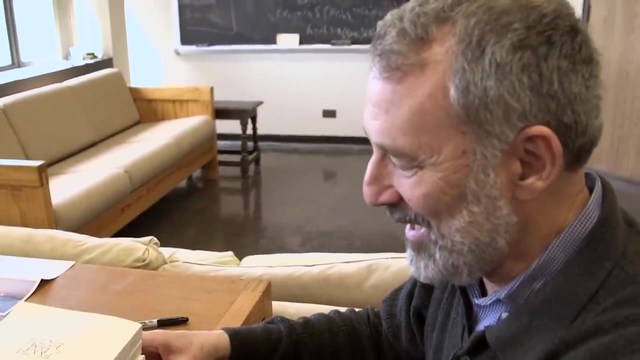 in my office, but I have lots of issues of the annals of mathematics. You have lots that you have. Oh yes, I have lots and lots and lots. So we're going to use copies of the annals of mathematics as dominoes. Let's just take two of them first. If I move this one here, it's going to collapse. 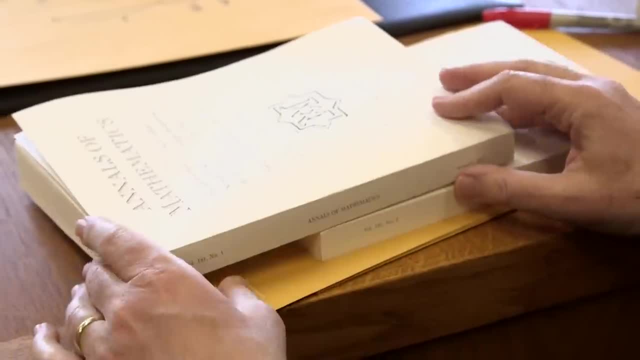 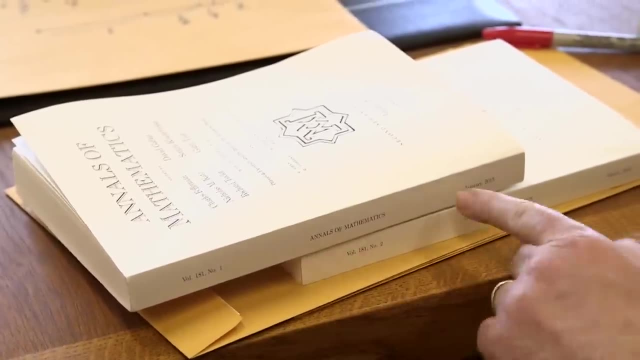 But if I move it so that its center of gravity is- Let's see if that works- I'm being a little conservative- The center of gravity of this guy is sitting over that guy, and so it does not collapse. Now let's take these two and put them very carefully on top. 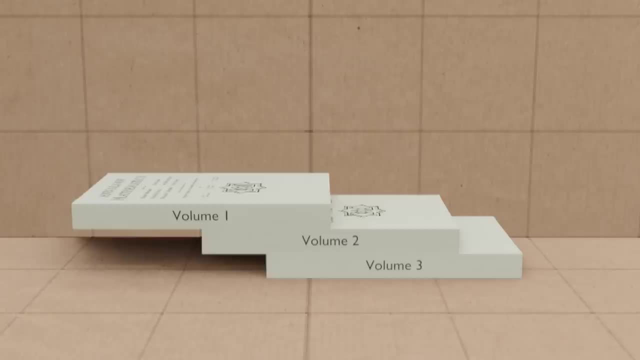 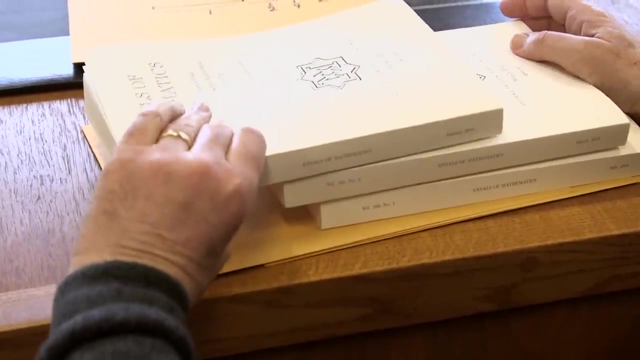 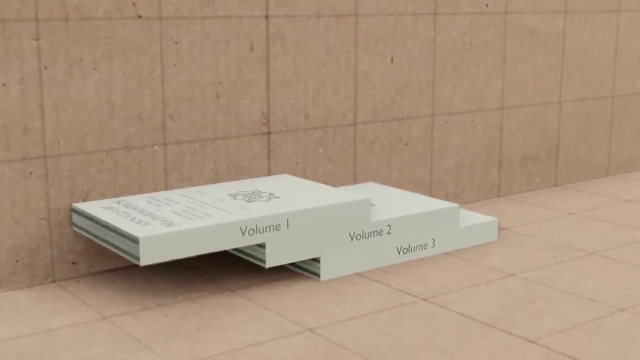 of the third one, taking care that the center of gravity of this whole guy is above this issue of the annals of mathematics, and therefore This looks precarious. Okay, there, It does not collapse. And now perhaps I could put these three on top of a fourth. and if I succeed in doing that, 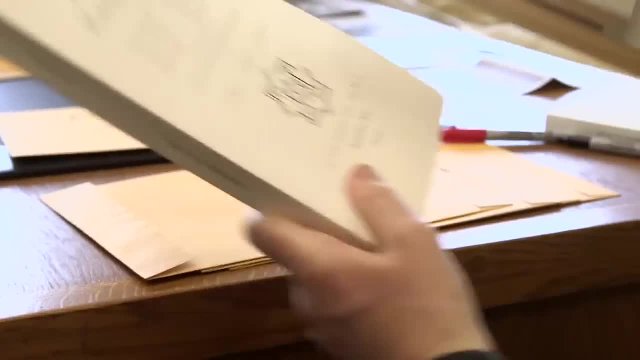 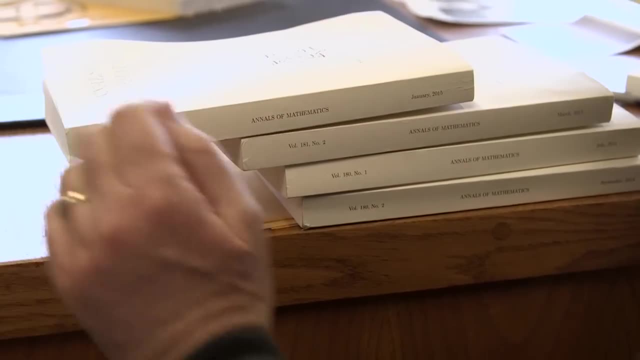 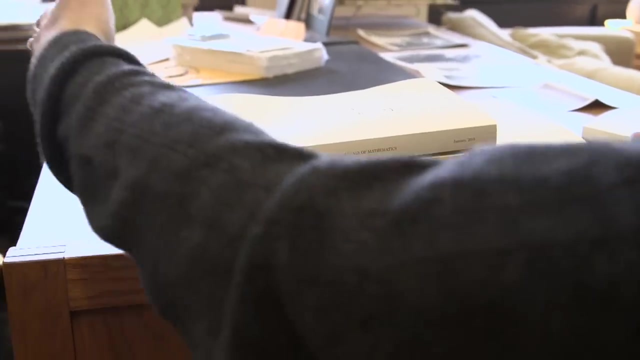 I will not tempt fate, I will just declare that we have succeeded. So let's see How are we doing. It hasn't collapsed. Looks a little flaky. It hasn't collapsed. How far can we make this guy stick out? Suppose that I have all those copies of the annals of mathematics, or perhaps all the 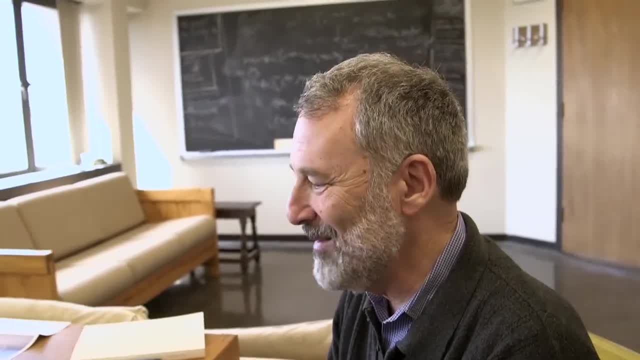 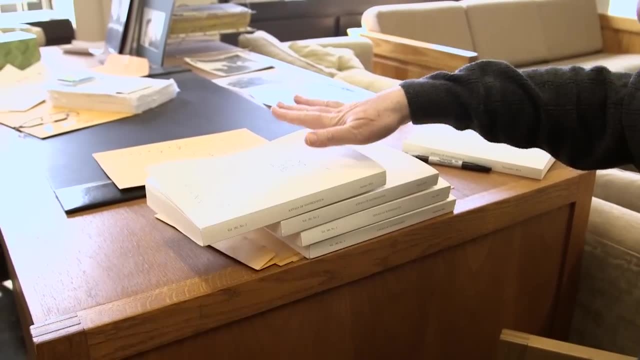 copies of the annals of mathematics ever printed, from the beginning of time to the end of time. Wonder how many that will be? Anyway, we have all of them and we stack them up and we demand that this pile cannot collapse. Well, this is merely paper, so sooner or later, if there's too much of 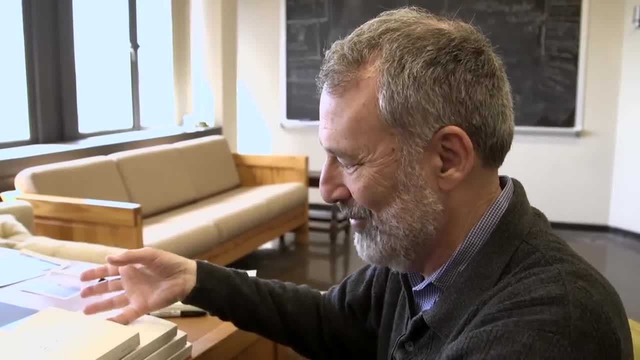 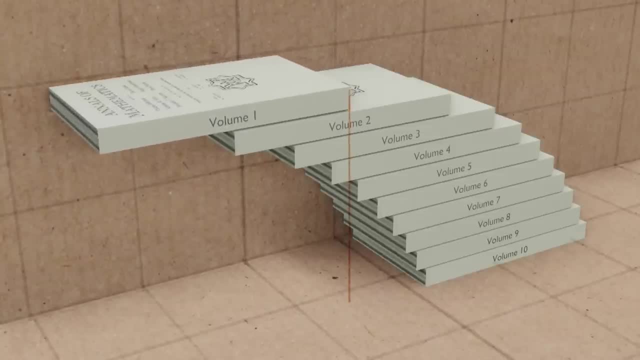 a load. it will be crushed, But never mind. These are imaginary rigid dominoes. Can we ever make the top guy so far out that it is not resting on the bottom guy at all, that this edge is not lying at all over this book but has come out farther, Further out in the bottom book? 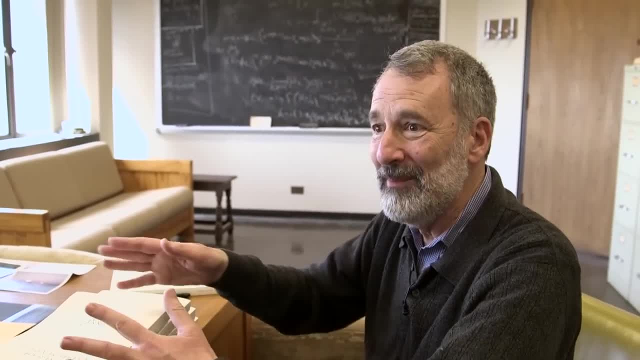 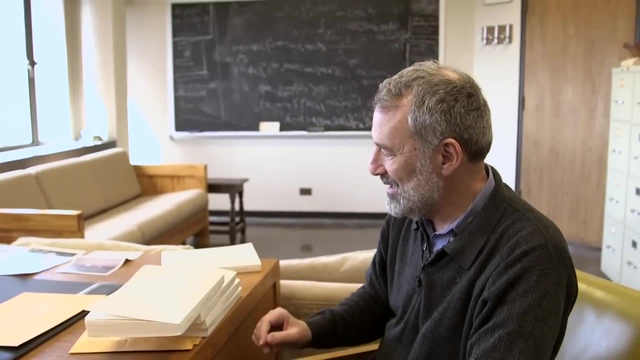 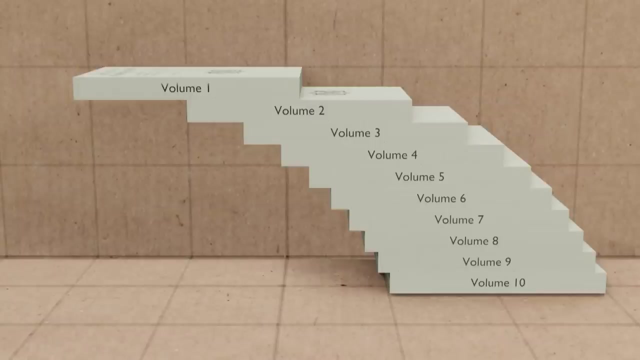 Exactly? And the answer is: oh, yes. In fact, you can make this, this pile, come out in that direction as far as you like, because if you look at it, if you have n copies of the annals of mathematics and you do an absolutely perfect job in an ideal world, the distances that they are slid out from 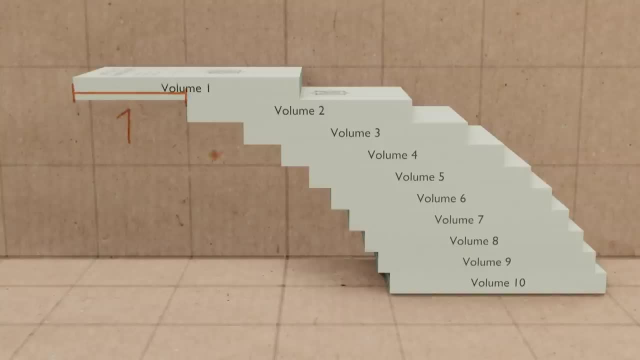 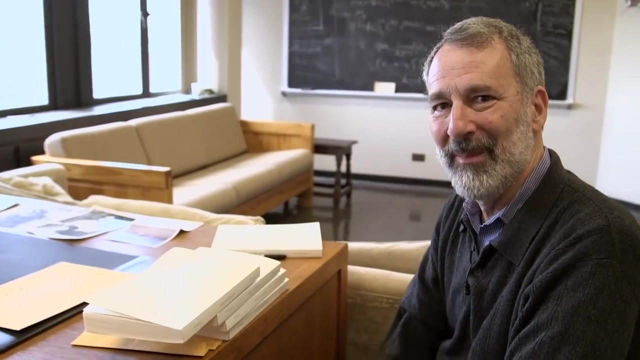 one another are in the proportions one to a half, to a third, to a fourth, to a fifth, to a sixth and so on, to one over n if there are n copies of the annals of math, or maybe n plus one copies of the annals of math. And so the fact that the harmonic series 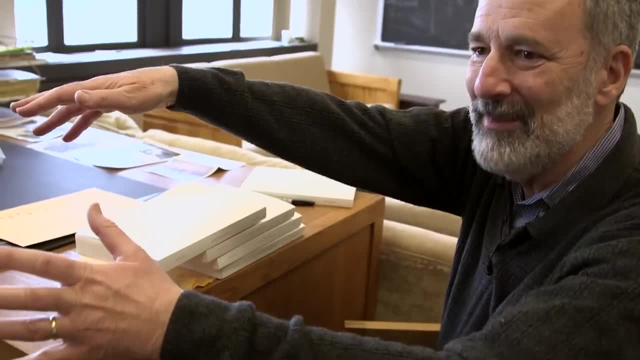 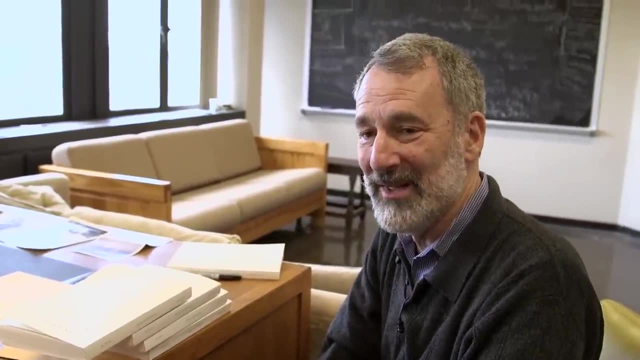 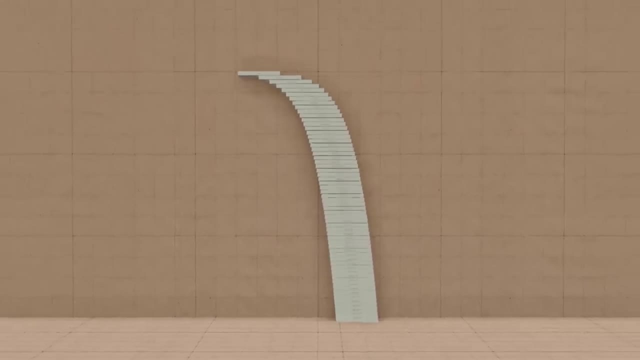 diverges, tells you that you can eventually make this pile come out as far as you like, because one plus a half, plus a third plus a fourth plus and so on. if you stop way way far out, after a gazillion- for a large enough value of a gazillion- will be more than 50 billion, And 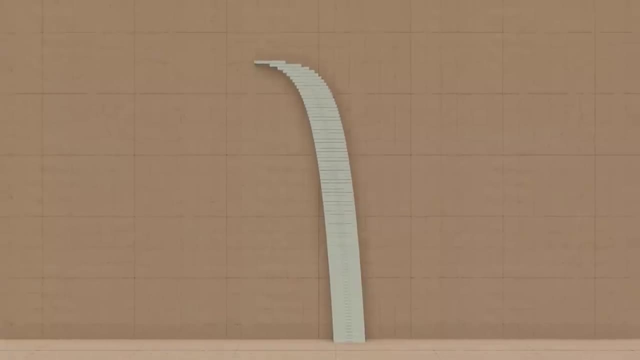 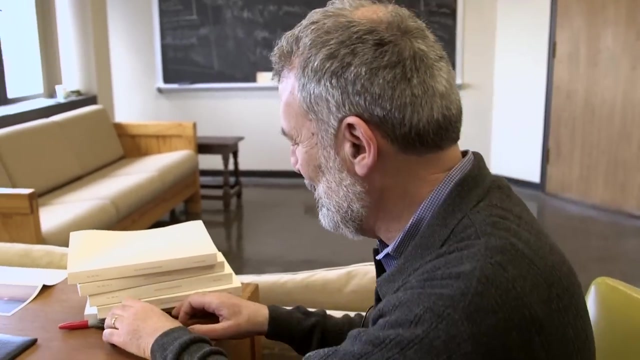 therefore, this distance out there will be more than 50 billion times the height of the annals of mathematics. All right, let's put the annals of mathematics aside Now. let's do the same thing to get the whole picture together. so I'm going to write it down, And so, basically what looks? 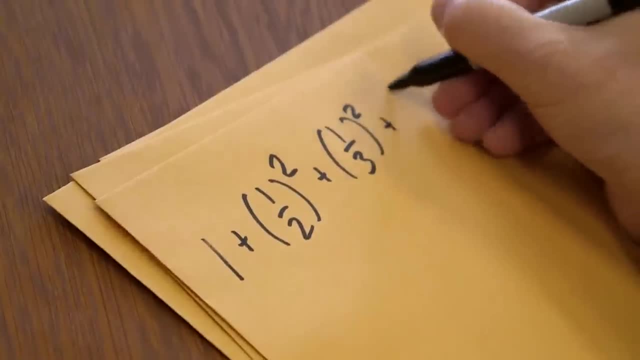 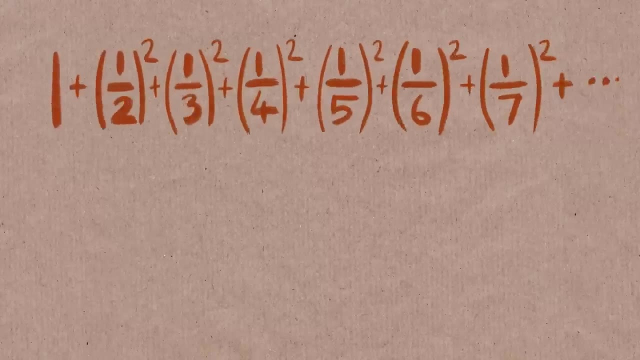 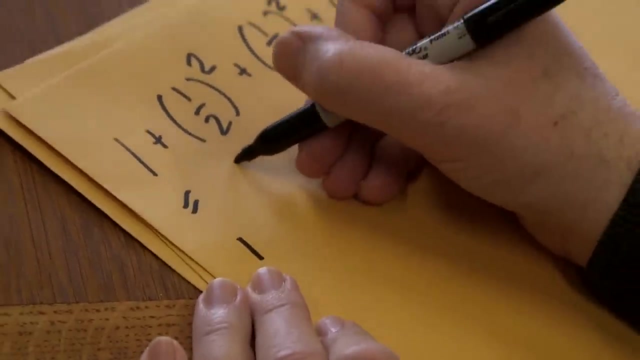 like it's an WITHIN procedure, We'd like to create a random loop of n of any discrete series: n plus one half squared plus n, plus the series n plus one half squared plus one third squared plus one fourth squared plus- let me keep going- one fourth squared, okay, blah, blah. Now let's. 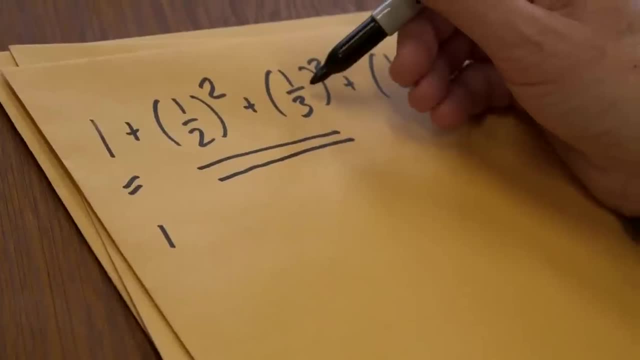 try to do the same thing. We're going to take the first term, all right, so that's one, thank you. Let's look at the next two terms smaller than one over a half squared. So we've got two terms and they're each smaller than. 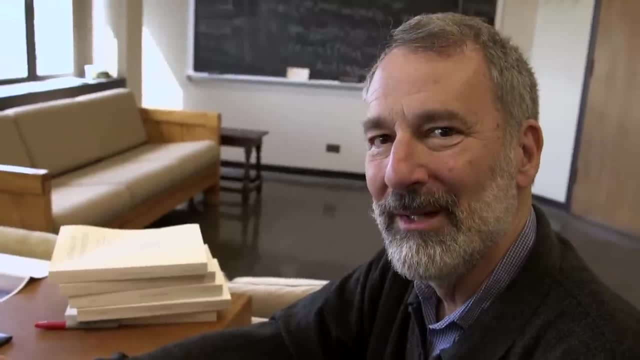 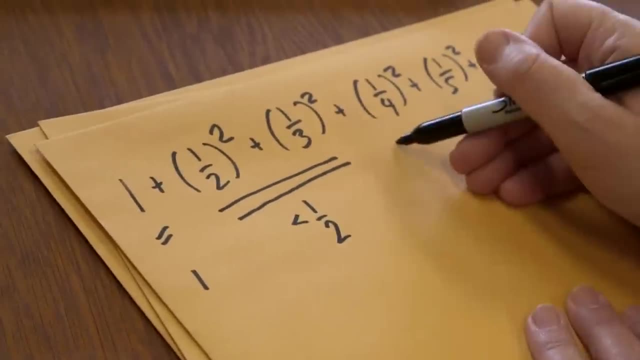 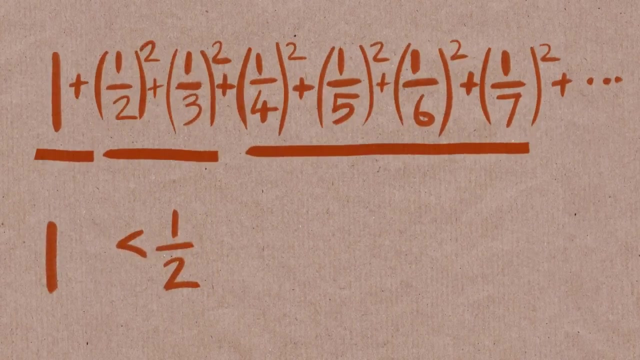 one half times one half. So that's smaller than two times a half times a half- That's smaller than a half. Let's look at the next four terms. Here they are. They're all one over four squared or smaller, So they're smaller than one fourth squared plus one fourth squared. 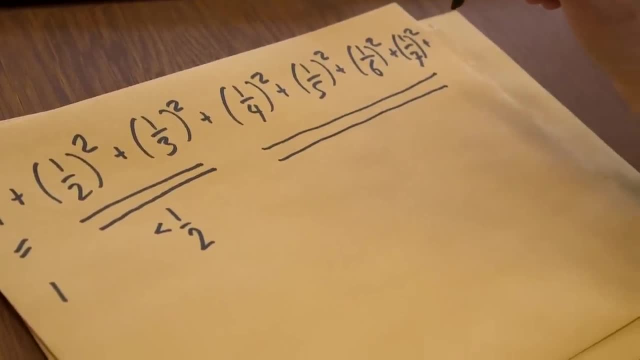 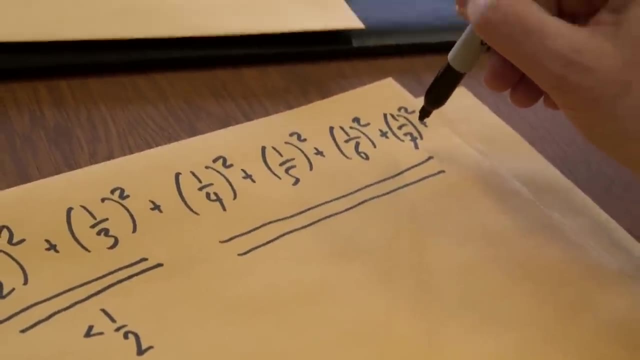 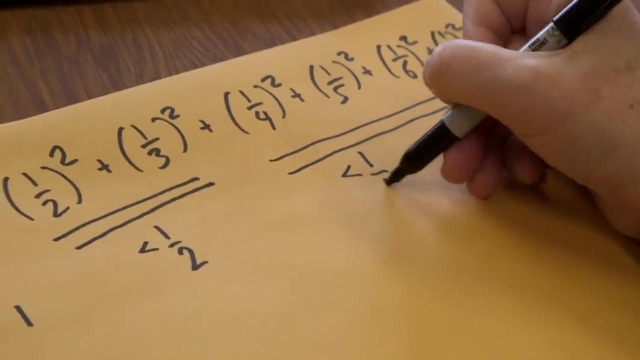 plus one fourth squared, plus one fourth squared. There are four terms there, and so these guys together are no bigger than four times one fourth squared. That's four times one, fourth times one fourth and that's one fourth. So this whole thing is less than one fourth. If I looked at the next, 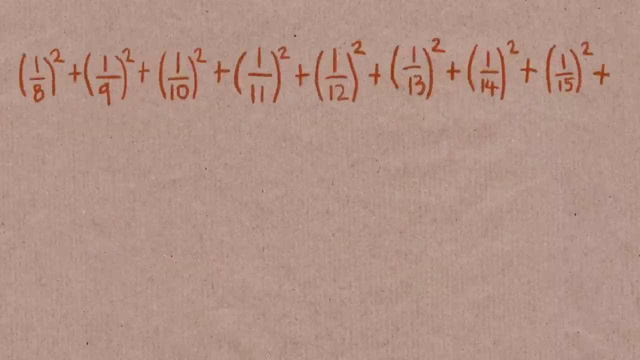 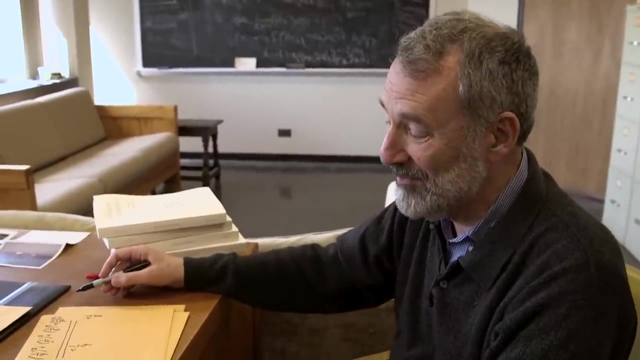 eight terms and played the same game, I would find that that's less than one eighth, and so on. So now look, if I go out to a gazillion terms, I'm guaranteed that what I've got is one over a half. What I've got is less than one plus a half, plus a fourth, plus an eighth, plus a sixteenth plus.